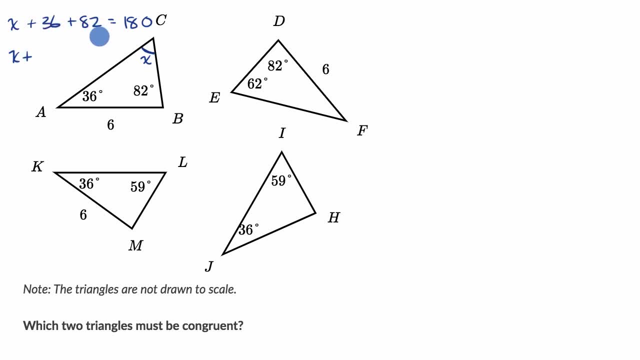 36 plus 82 is 118.. Did I do that right? Six plus two is eight, And then three plus eight is 11.. Yep, that's right. So that's going to be equal to 180.. And then, if I subtract 118 from both sides, 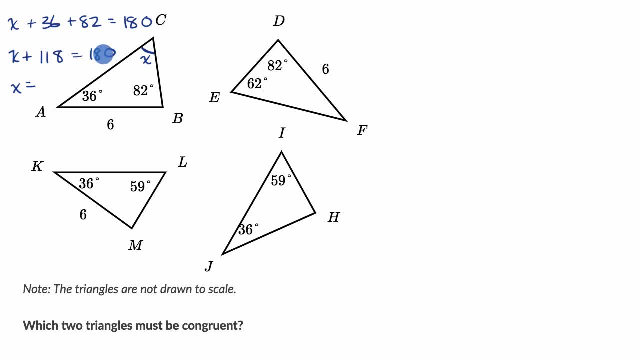 I'm going to get. X is equal to 180 minus 18 is 62. So this is X is equal to 62, or this is a 62-degree angle. I guess is another way of thinking about it. I could put everything in terms of degrees if you like. 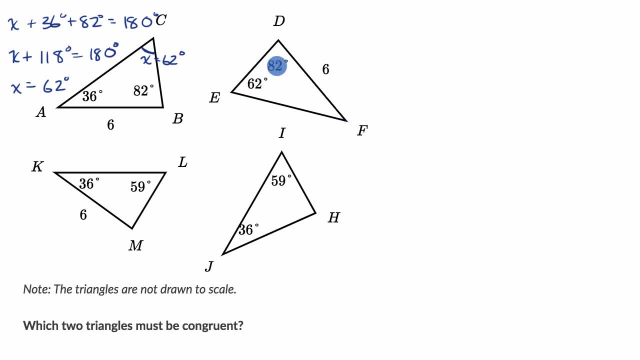 All right, now let's do the same thing with this one right over here. Well, this one has an 82-degree angle and a 62-degree angle, just like this triangle over here, But the third angle needs to be 36 degrees, 36 degrees. 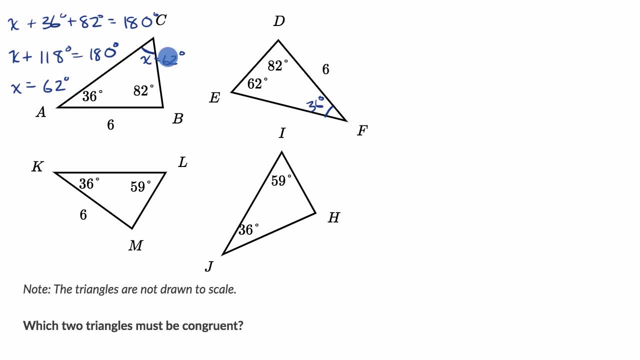 because we know 82 and 62, if you need to get to 180, it has to be 36.. We just figured that out from this first triangle over here. Now, if we look over here, 36 degrees and 59,. 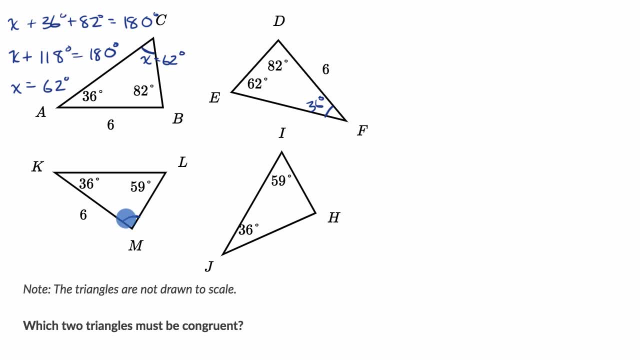 this definitely looks like it has different angles, but let's figure out what this angle would have to be. So if we call that Y degrees, we know I'll do it over here- Y plus 36.. 36 plus 59 is equal to 180.. 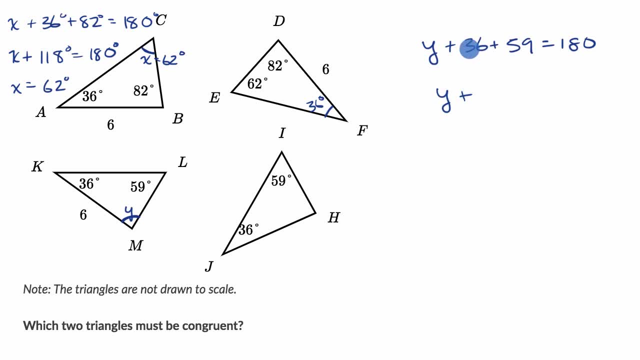 And I'm just thinking in terms of degrees here. So Y plus this is going to be equal to what is this? This is going to be equal to? 95 is equal to 180.. Did I do that right? Yep, that's 80 plus 15,, yep, 95.. 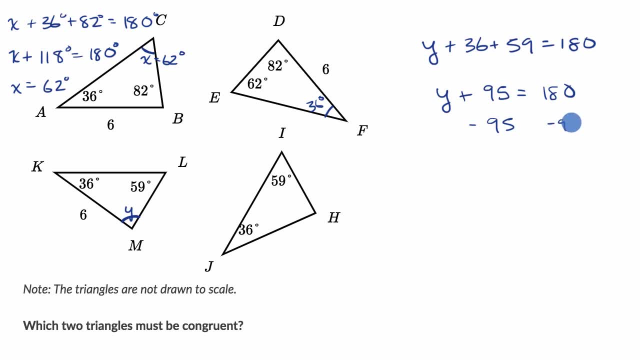 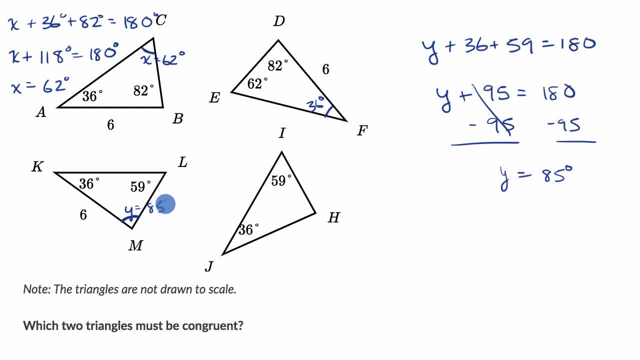 I'm left with. Y is equal to 85 degrees, And so this is going to be equal to 85 degrees, And then this last triangle right over here I have an angle that has measure 36, another one that's 59.. 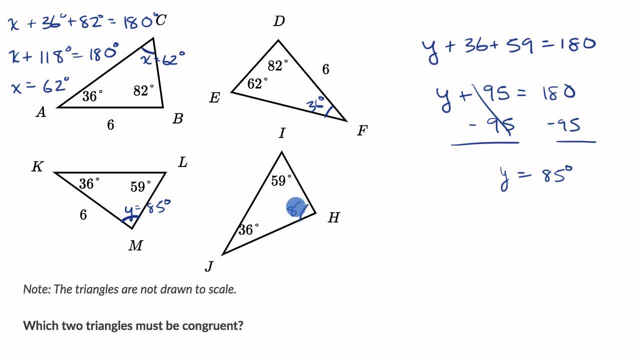 So, by the same logic, this one over here has to be 85 degrees. So let's ask ourselves, now that we've figured out a little bit more about these triangles, which of these two must be congruent. So you might be tempted to look at these bottom two triangles.